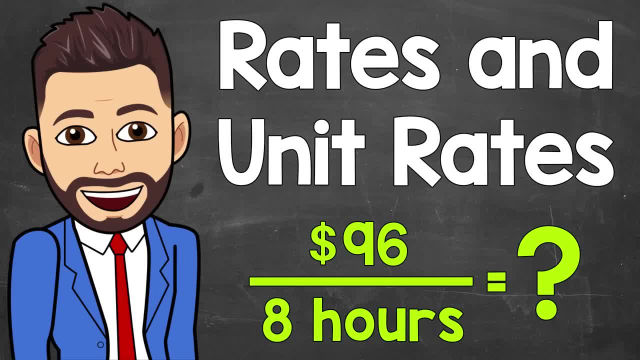 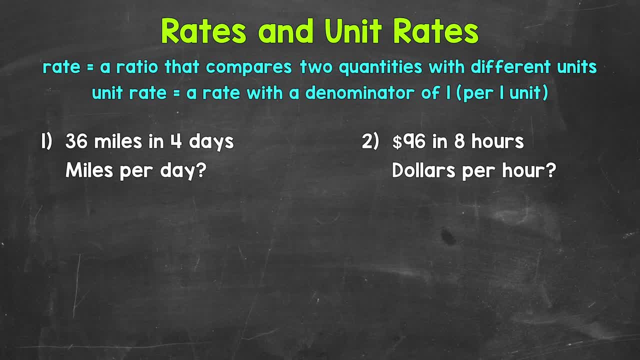 Welcome to Math with Mr J. In this video I'm going to cover the basics of rates and unit rates. I'll cover what rates and unit rates are and then how to find unit rates. Now, rates compare and show the relationship between quantities with different units. 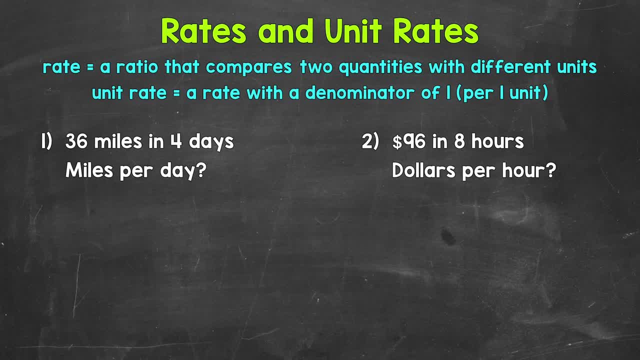 So rates are just ratios that compare and show the relationship between quantities with different units. A unit rate is a specific type of rate. A unit rate is a rate with a denominator of 1. It shows per one unit. Let's jump into our examples and see exactly what this means. 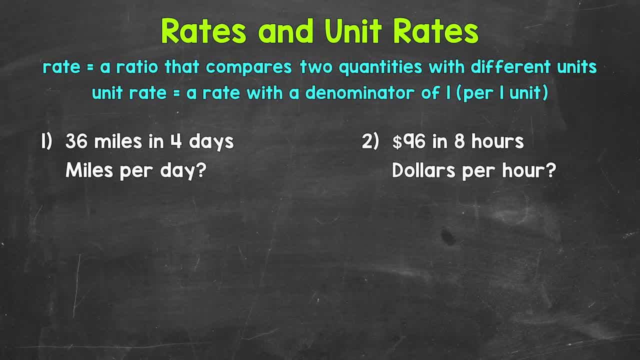 Starting with number 1, where we have 36 miles in 4 days. For example, let's say that someone rode their bike 36 miles in 4 days. This rate compares and shows the relationship Between the number of miles ridden and the days that it took to do so. 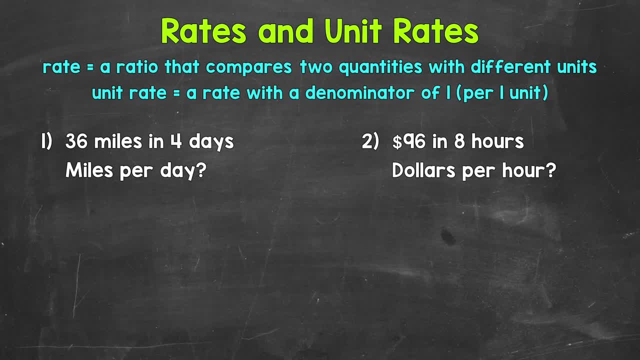 So two different units of measure, miles and days. We can write this rate as a fraction. Now order matters. We have miles and then days, So our fraction needs to represent that order: 36 miles in 4 days. Make sure to label and include units within rates, since we are working with different units. 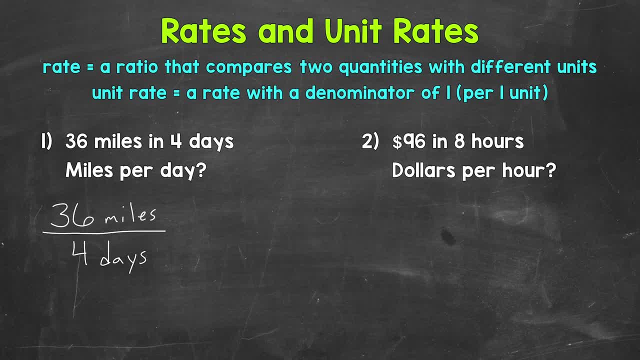 We need to be clear what those units are. So this is a rate: 36 miles in 4 days. Now let's find the unit rate. Unit rates always have a denominator of 1.. We want per one unit In this case. we want how many miles per one day? 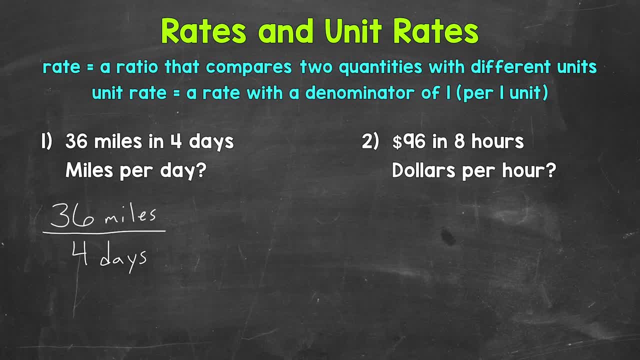 Let's do this by dividing our denominator by 4.. That will give us a denominator of 1, representing one day. So 36 miles in 4 days is going to equal. Well, again, we need to divide by 4 in order to get that denominator of 1.. 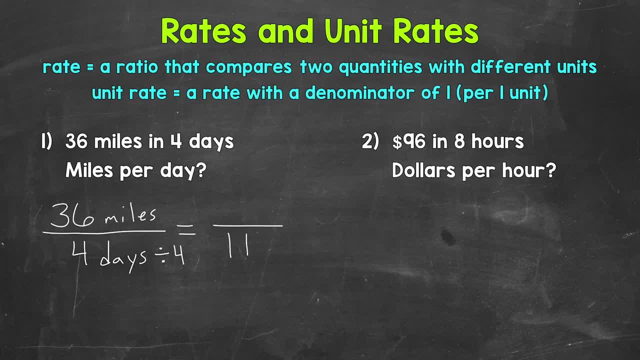 4 divided by 4 is 1, and we need to label. so this is one day: Whatever we do to the bottom, we must do to the top. So divide 36 by 4 as well. 36 divided by 4 is 9.. 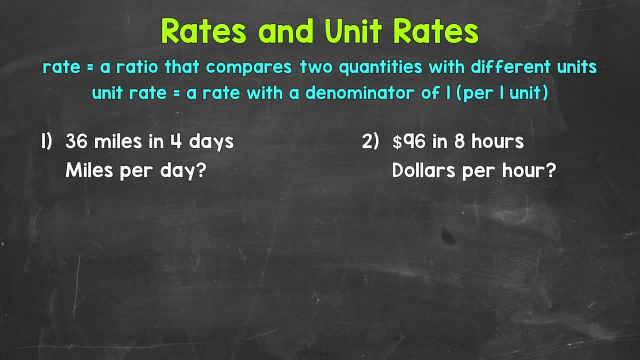 So two different units of measure, Miles and days. We can write this rate as a fraction. Now order matters. We have miles and then days, So our fraction needs to represent that order: 36 miles in 4 days. 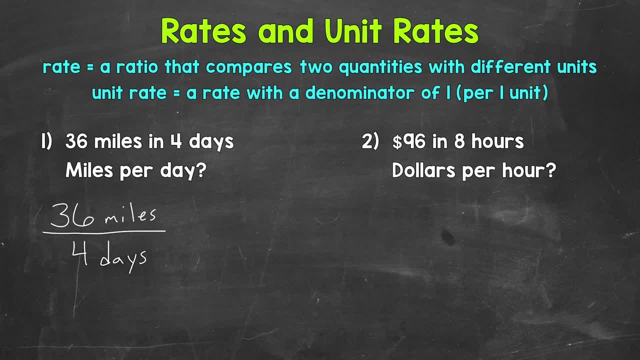 Make sure to label and include units within rates. Since we are working with different units, we need to be clear what those units are. So this is a rate: 36 miles in 4 days. Now let's find the unit rate. 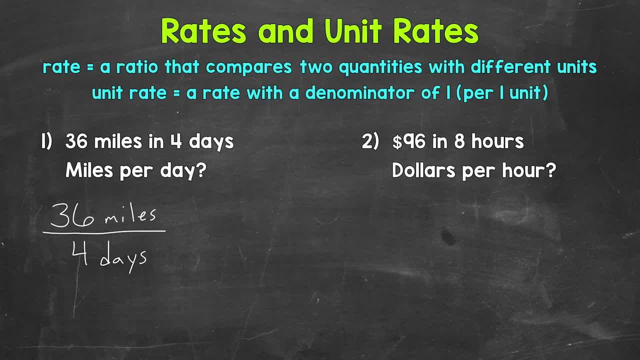 Unit rates always have a denominator of 1.. We want per one unit. In this case, we want how many miles per one day. Let's do this by dividing our denominator by 4.. That will give us a denominator of 1, representing one day. 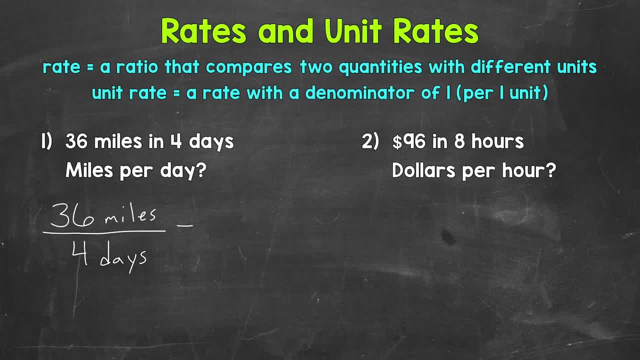 So 36 miles in 4 days is going to equal. Well, again, we need to divide by 4 in order to get that denominator of 1.. 4 divided by 4 is 1, and we need to label. 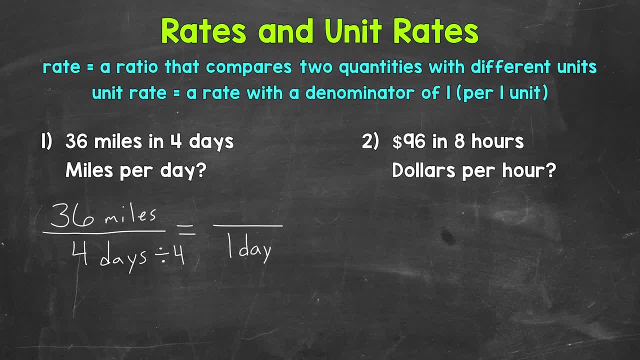 So this is one day: Whatever we do to the bottom, we must do to the top. So divide 36 by 4 as well. 36 divided by 4 is 9.. And this is miles, And that's our unit rate. 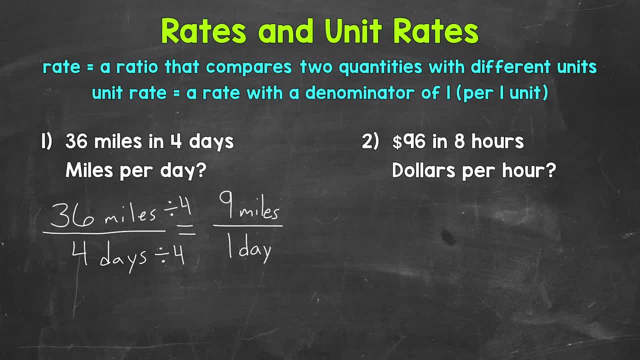 9 miles per one day or 9 miles per day. Now we can also write this as 9 miles per day. So our original rate was 36 miles in 4 days, And then we found our unit rate. We did that by getting our denominator to equal 1.. 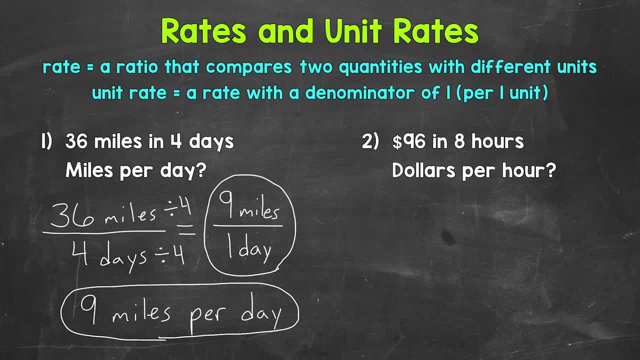 We did that by dividing by 4.. That gave us 9 miles per day. Let's move on to number 2, where we have $96 in 8 hours. So someone makes $96 in 8 hours. We will write that as a rate in fractional form and then find the unit rate. 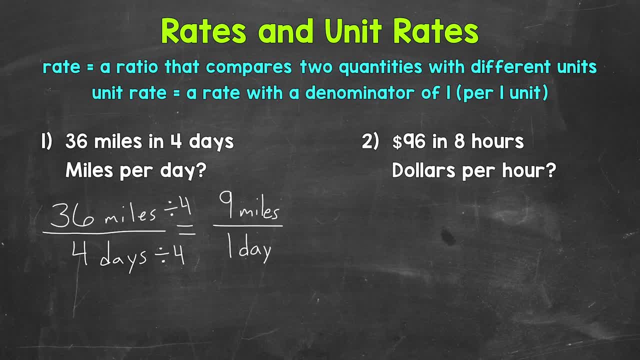 And this is miles And that's our unit rate: 9 miles per one day or 9 miles per day. Now we can also write this as 9 miles per day. So our original rate was 36 miles in 4 days. 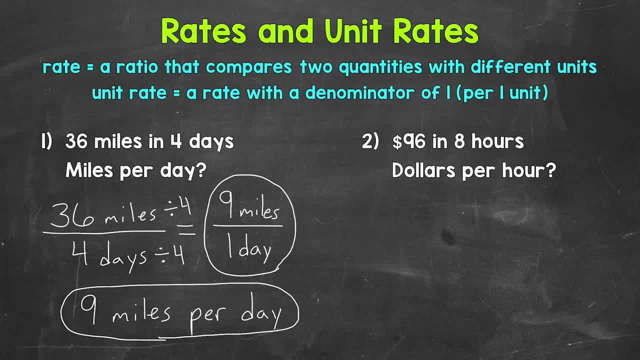 And then we found our unit rate. We did that by getting our denominator to equal 1.. We did that by dividing by 4.. That gave us 9 miles per day. Let's move on to number 2, where we have $96 in 8 hours. 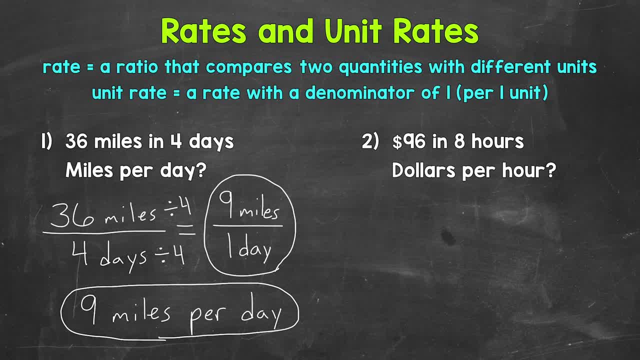 So someone makes $96 in 8 hours. We will write that as a rate, Write that as a rate in fractional form And then find the unit rate. So let's first write that as a rate in fractional form, So we have $96 in 8 hours. 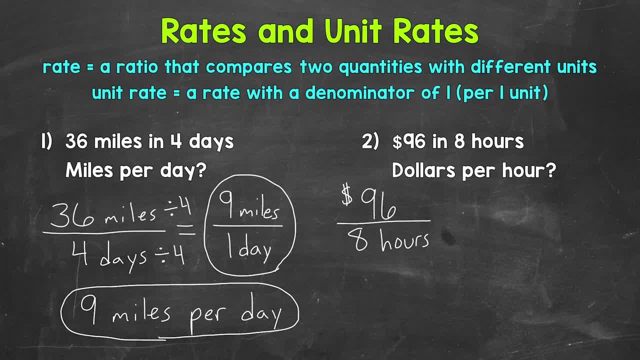 So that's our rate. Let's find our unit rate. So how much money per 1 hour? We can do this by dividing by 8. Because again we need that denominator to equal 1. So let's divide by 8 here to give us 1 hour. 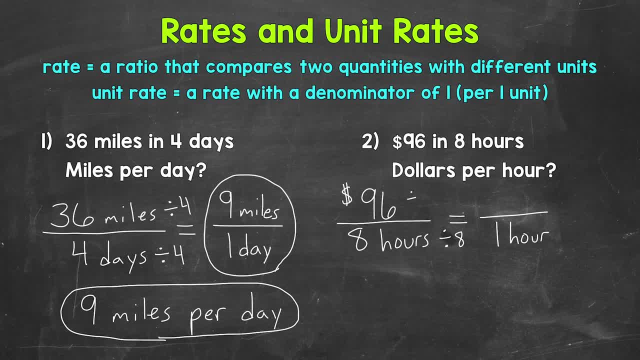 Whatever we do to the bottom, we must do to the top. So 96 divided by 8 as well, That gives us $12.. So our unit rate is $12 per 1 hour or $12 per hour. We can also write that as $12 per hour. 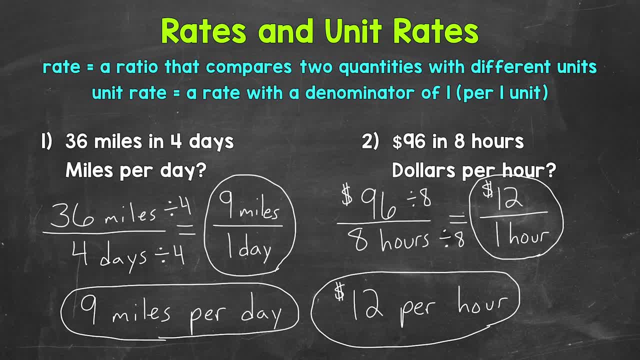 So there you have it. There's how you write rates and unit rates. Rates are ratios that compare two quantities with different units, And then a unit rate is a specific type of rate. It's a rate with a denominator of 1.. We show per 1 unit. 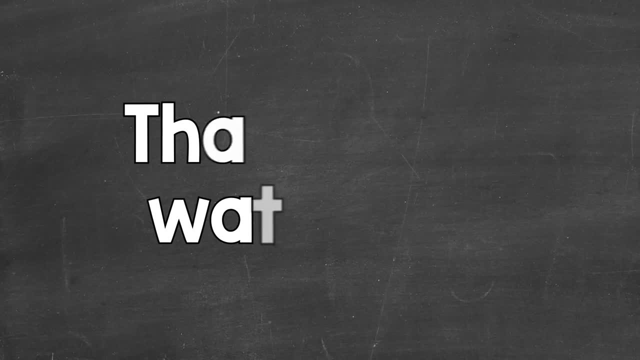 I hope that helped. Thanks so much for watching. Until next time, Peace.